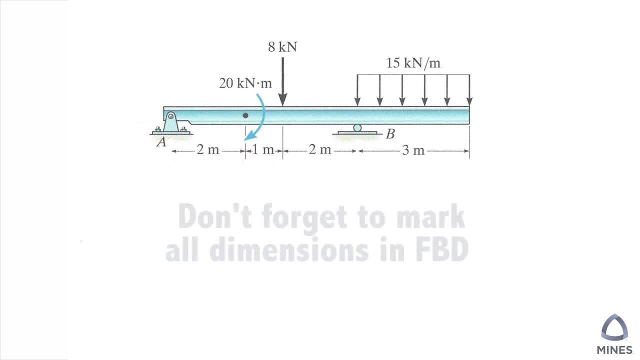 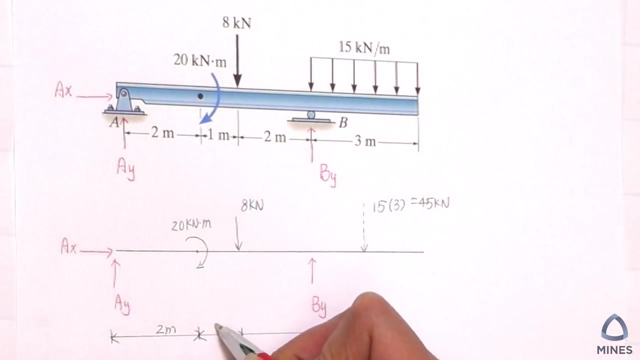 thing you have to do is try to mark all the dimensions so that you can. you will be ready to write down all the equilibrium equations So we can see. the moment is acting 2 meters away from A point, and 8 kN is a little bit further than the dimension for the EY. So now what we have to do is try to mark where is the simplifier? 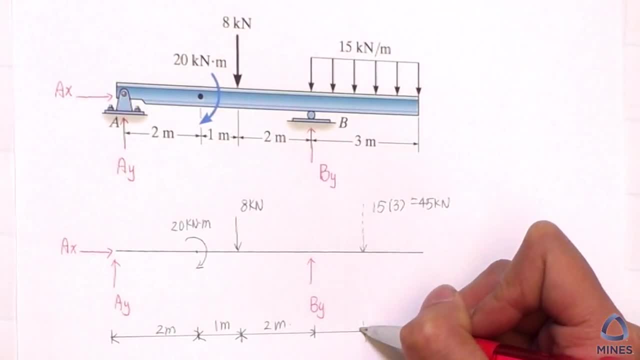 the total force for the uniformly distributed load. This is a triangle distributed load, which means it will pass through the centroid, which will be 1.5 meters from the beam. So, after you include all the forces for the dimension, which means you are ready. 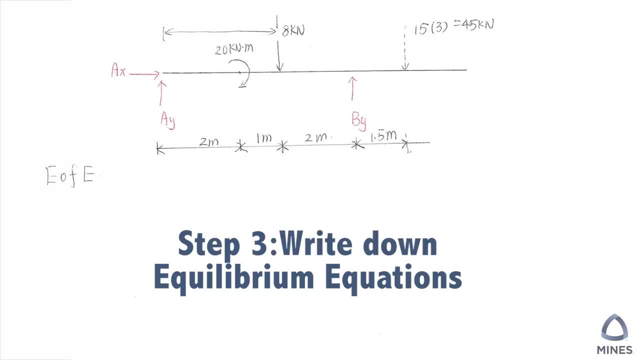 to write down the equilibrium equations. So most of the time, what we are going to do is trying to summarize moment around the most unknown forces. so which will be the A point for our case? and counterclockwise moment will be positive. So now let's summarize. 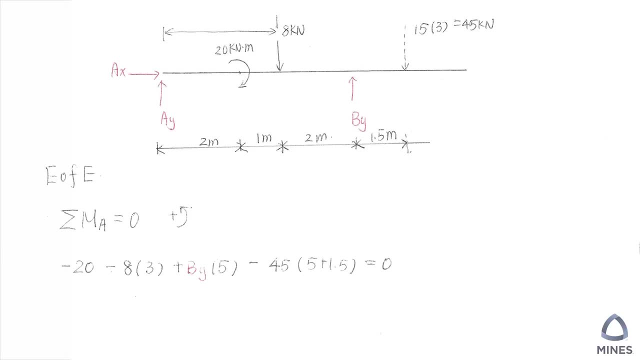 So we had 20 kN but clockwise negative. and then we can see: for the 8 kN. here it will create a moment. It's a clockwise moment, so we put a negative sign. So force times the distance, so the distance. 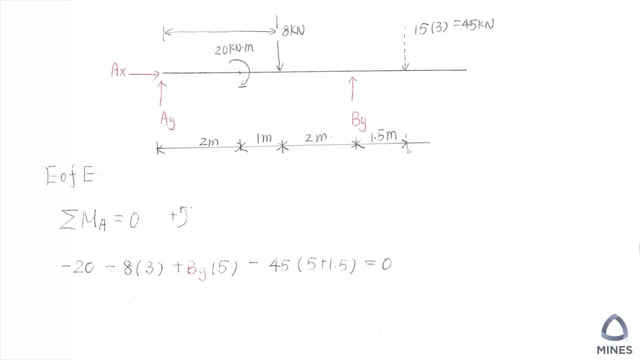 from 8 kN to A point will be 3 meters. And then we had- we just keep moving. we had BY multiply the total length, that's going to be 5, and then we still had simplified, uniformly distributed load: 45, multiply the. 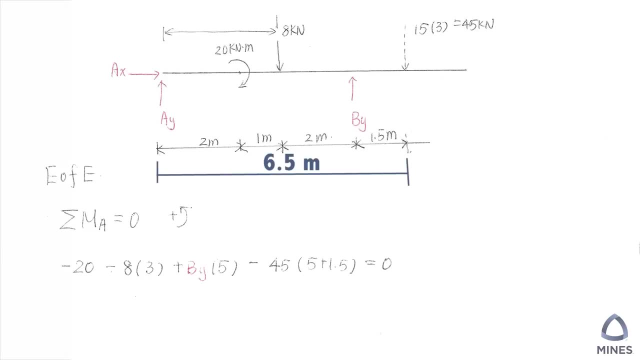 length to the A, which will be 5 plus 1.5.. So once you've done every load, everything summarized to the zero in this equation, you can see we had one unknown force. so which means we can find the BY is equals to 67.3 kN and it's 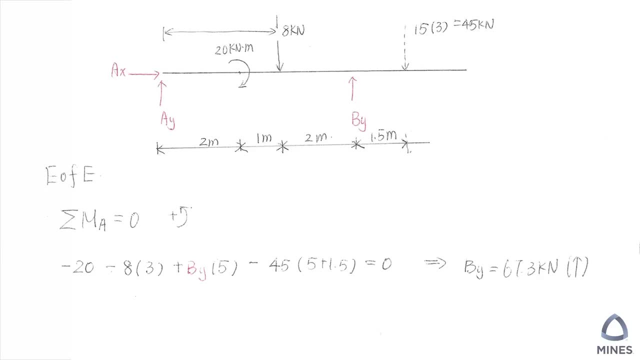 positive, which means our assumption go up is correct. So after you find the BY, which means if we summarize the force in the Y direction, we should be able to find out what is AY And we can also try to summarize the force.